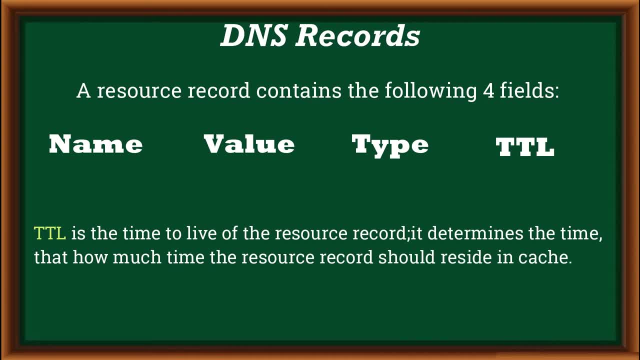 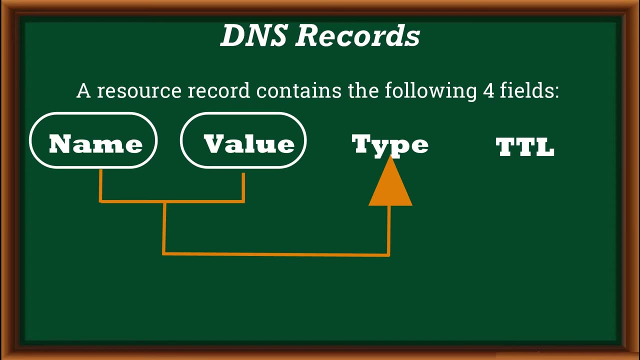 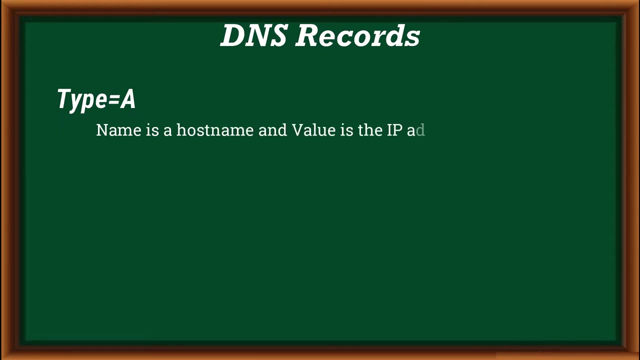 Here TTL is the time to live of the resource record. It determines the time, that how much time the resource record should reside in cache. The meaning of name and value field depend on the type field here. If a type is equal to A, then name is a host name and value is the IP address for the host name. 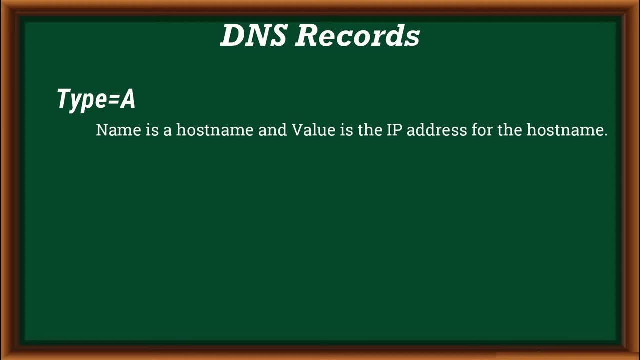 Thus a type A record is a resource record. The second field name provides the standard host name to IP address mapping, For example relay1.foocom, and IP address for relay1.foocom is 145.37.93.126.. That is a type A record. 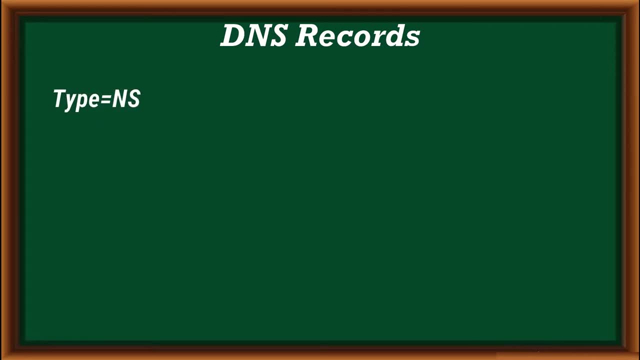 If type is equal to NS, then name is a domain name, such as in the above example. Foocom is a domain name and value is the host name of an authoritative DNS server that knows how to obtain the IP addresses for host in the domain. 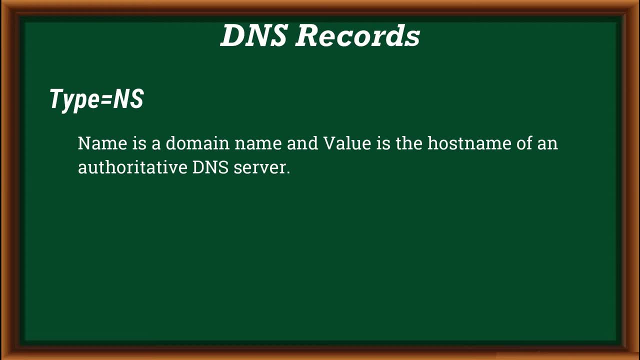 This record is used to route DNS queries further along in the query chain. As an example, foocom and dnsfoocom is a type NS record. If type is equal to CNAME, then name is a domain name, such as in the above example. 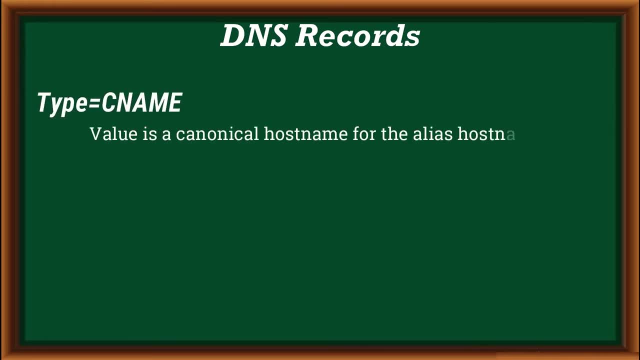 If type is equal to MX, then value is the canonical host name for the alias host name. This record can provide querying host the canonical name for a host name. As an example, foocom- relay1.foocom is a canonical name record. 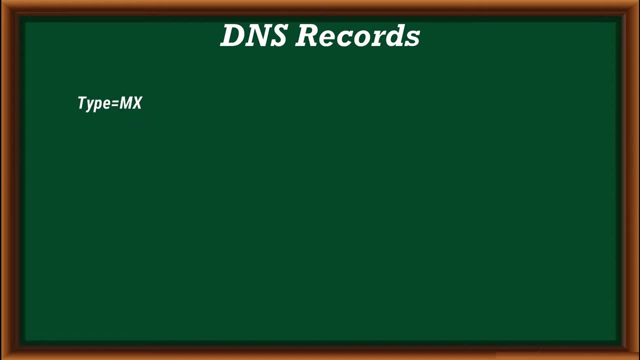 If type is equal to MX, then value is the canonical name of a mail server That is an alias host name, As an example foocom. then mailfoocom is an MX record. So these are all the DNS records. Now coming to the DNS messages. 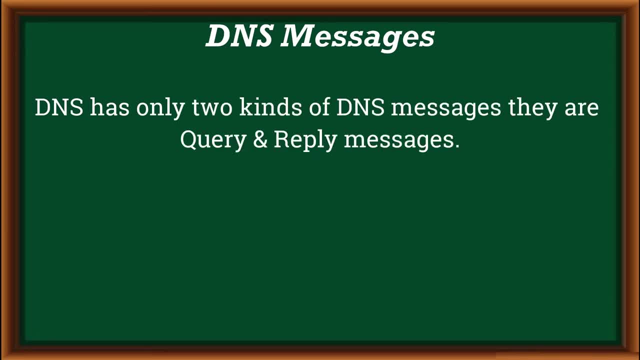 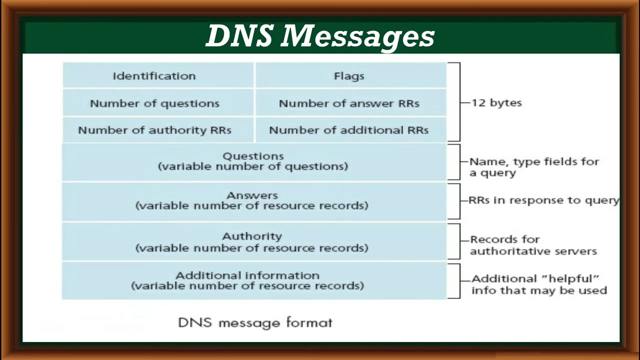 DNS has only two kinds of DNS message. They are query message and reply messages. Both query and reply messages have the same format as shown in this figure. The first 12 bytes is the header. This is the header section, which has a number of fields, as shown in the figure. 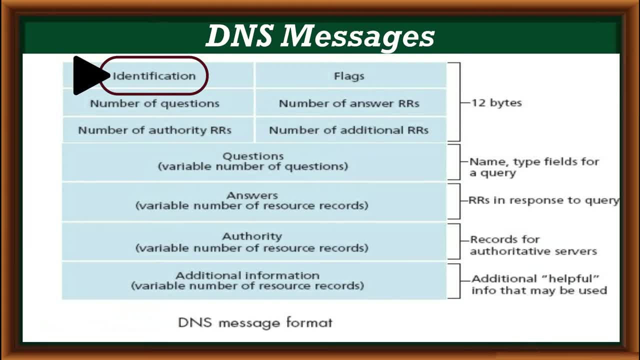 The first field is a 16-bit that identifies the query. This identifier is copied into the reply message to a query, allowing the client to match received replies with the sent queries. There are a number of flags in the flag field. A 1-bit flag bit indicates whether the message is a query message or reply message. 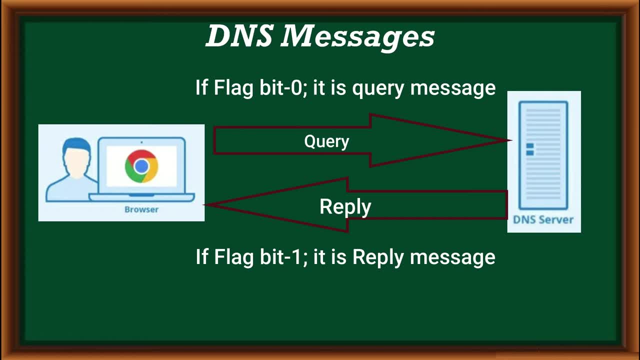 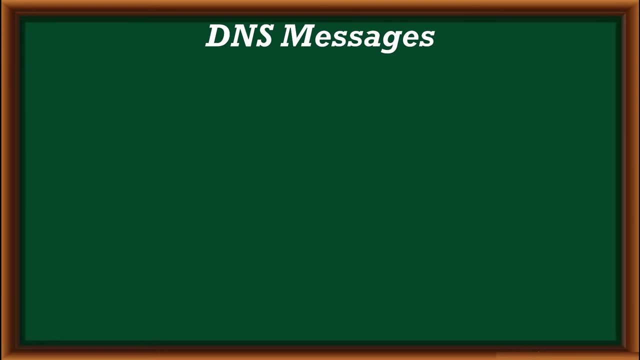 This is the flag field. If a flag bit is 0, it indicates a query message And if a flag bit is 1, it indicates a reply message. The question section contains information about the query. This section includes a name field that contains the name that is being queried and a type field. 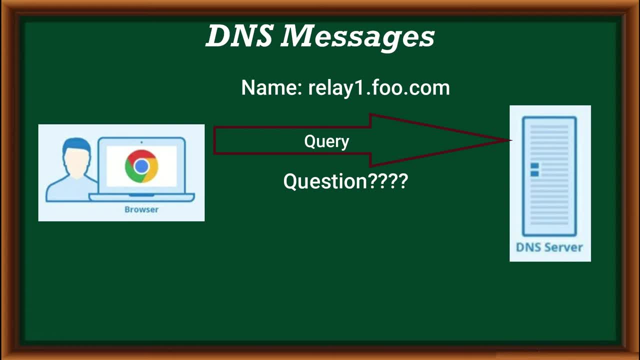 that indicates the type of question being asked about the name, For example, a host address associated with the name that is, for type a or type ns or type c name are the examples in a reply from the dns server. the answer section contains the resource records for the name that was originally queried, the 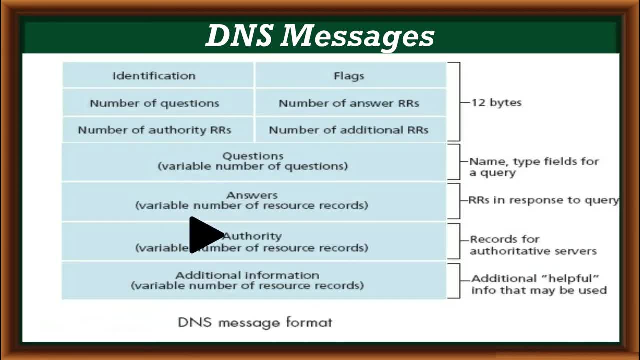 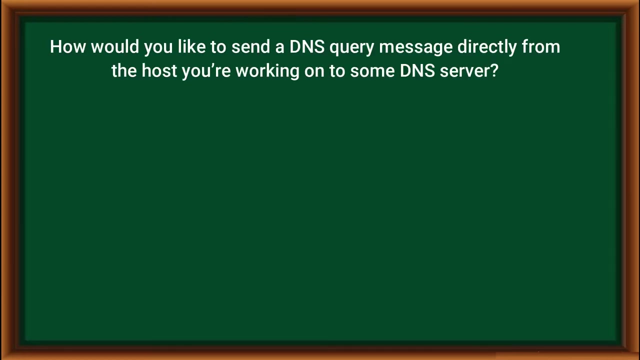 authority to section contains records of other authority to servers. the additional section contains other helpful records. for example, the answer field in a reply to an mx query contains a resource record providing the canonical hostname of a mail server. now let us see how. would you like to send a dns query message directly from your laptop or from your system which you are working? 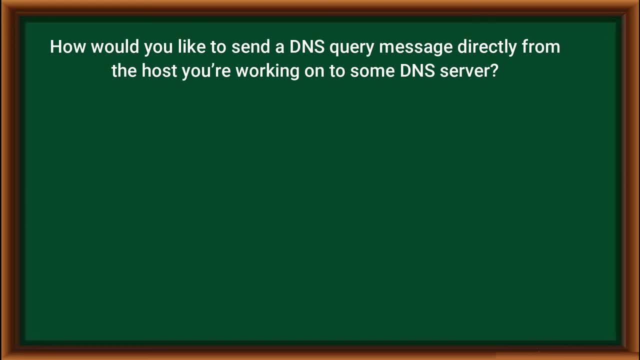 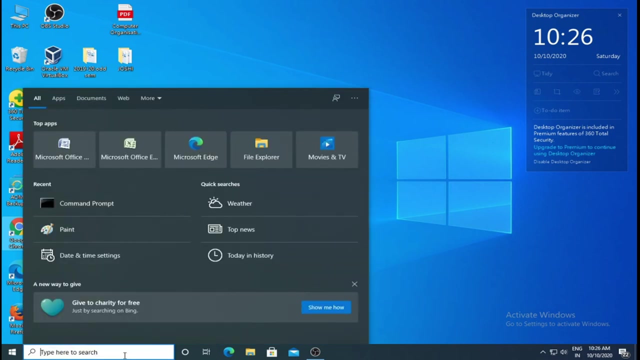 onto the some dns server. so this can be easily done with the command questions called nslookup program command, so which is available from most windows and unix platforms, for example from a windows host, to know the nslookup command. so what we need to do, we need to open the command prompt by typing a cmd command in windows operating system. 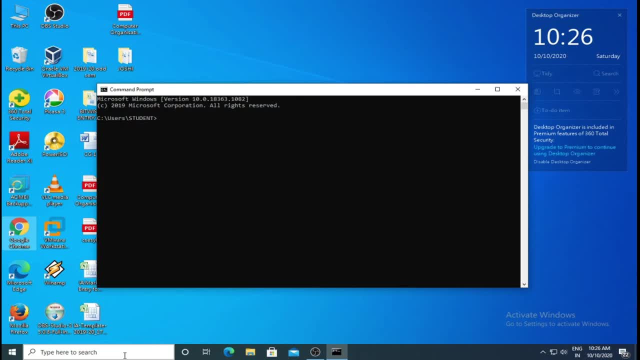 then here you need to type the nslookup command. so after executing this command i'll get the reply, as the default server is multiplybsnlin and the ip address of this dns server is 61.1.1.1. so this is my default dns server and the address of the dns server here. so whatever the request, 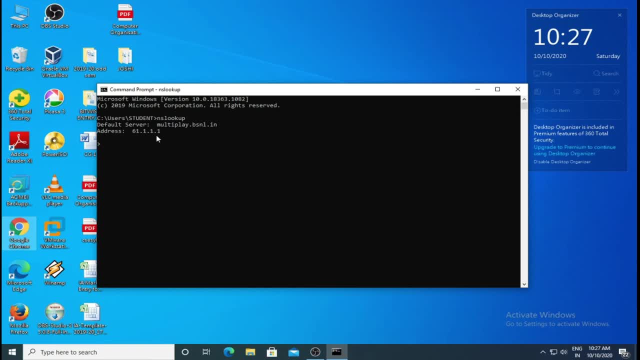 query message is sent to the dns server, it will be sent to the dns server and it will be sent to from this system. so first will be directed to this default dns server. so this is my default dns server, which is of multiplybsnlin. so this dns server, which maintains the 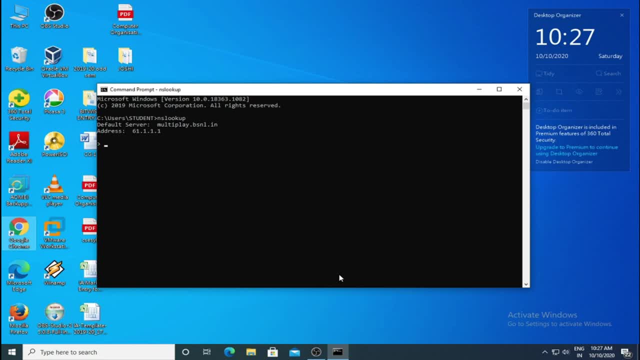 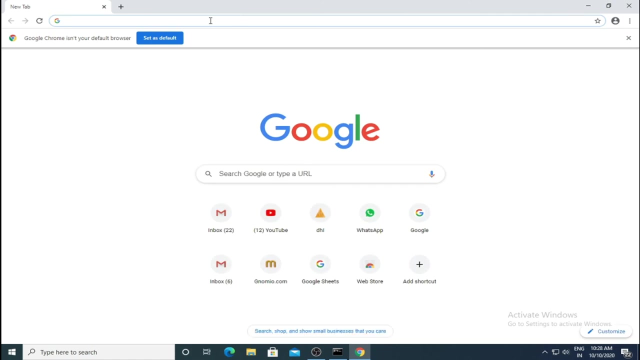 ip addresses of the host name here. so whenever my host request the ip address of the host name, then so first it will be directed to this dns server and this dns server will reply back with the requested host name ip address. suppose consider i opened. i want to visit the googlecom. 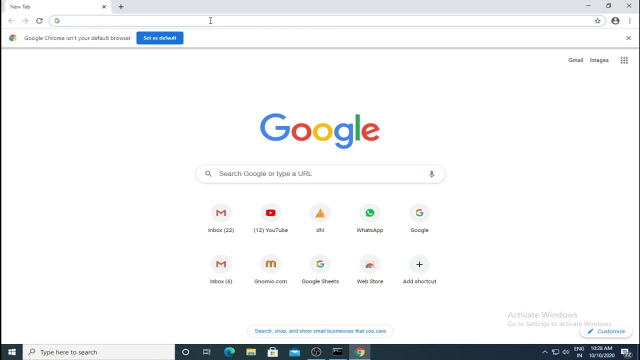 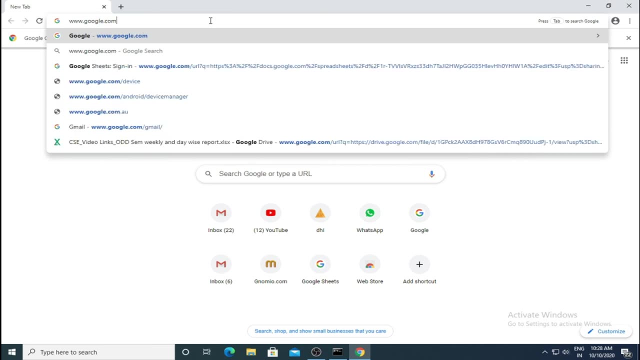 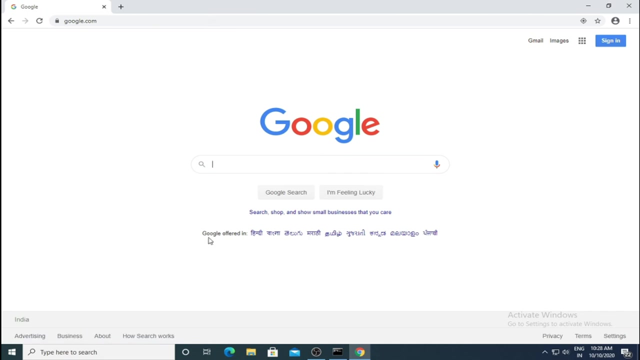 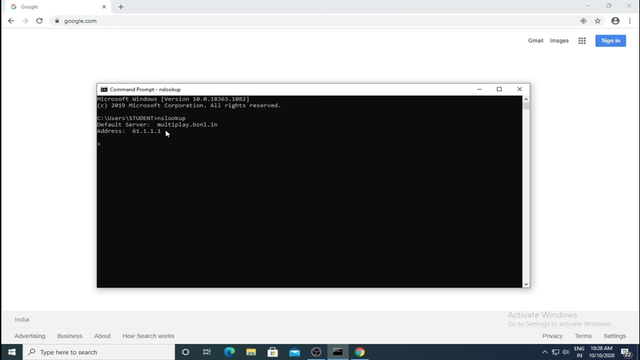 so what i will do? i will open a browser. then i will type the url as what: wwwgooglecom. right? so first my browser has to request the ip address of google server here. so my default dns server is what the multiplybsnlin which maintains. 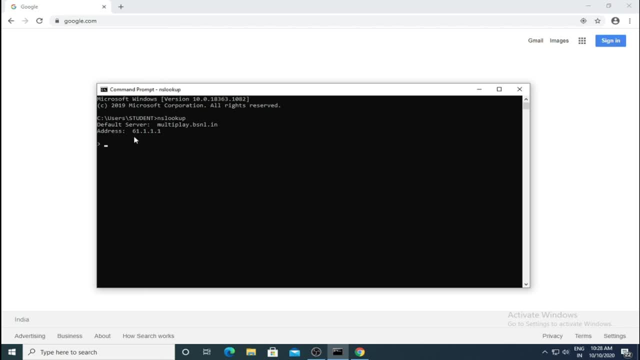 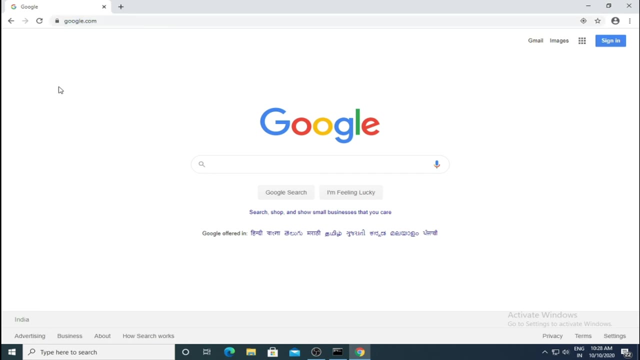 the ip addresses of all the host names here. so my first request will go to the dns server and the dns server will reply back the ip address of google server. then my browser will be able to establish a tcp connection with the google server. then it can send the http request message and 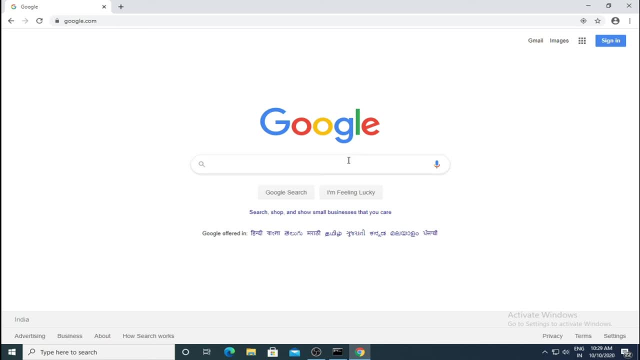 gets the http response message from the google server here. so this is how the dns works, thank you. thank you for watching this video.